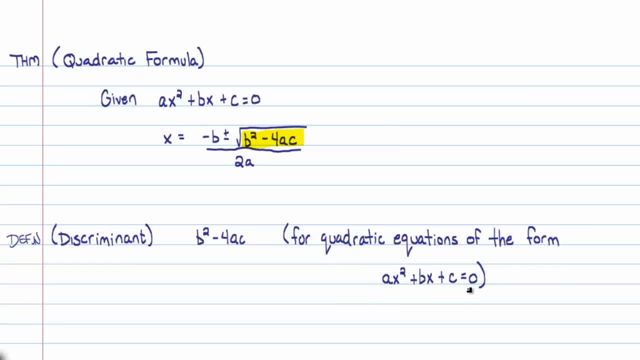 The reason why we want to label this specifically is because it allows us to determine the kind of solutions that our equation has. For example, suppose that in our quadratic equation, we have that b squared minus 4ac turns out to be positive. In other words, if you look at the quadratic formula, the stuff underneath the square root here is positive. What that essentially implies is that we have two real solutions. Not only do we have two real solutions, but there are two different real solutions. And that's because this equation is positive. 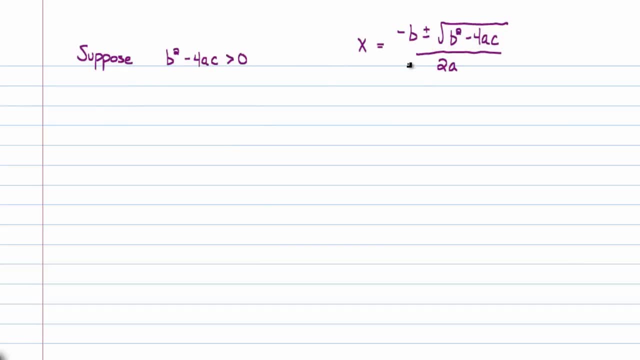 This number underneath the square root is positive, and it's greater than 0. So you have something like a negative 1 plus or minus the square root of 3 over 2, or something like that. We get two real solutions, negative 1 plus root 3 over 2 and negative 1 minus root 3 over 2. So this implies two real solutions. 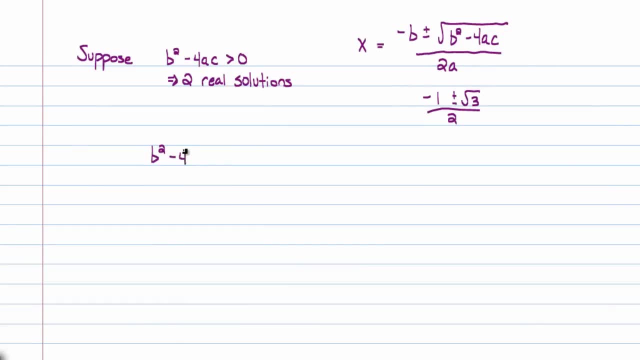 If on the other hand, b squared minus 4ac is actually equal to 0, well then, our solutions would be of the form negative b plus or minus the square root of 0 over 2. Or in other words, just a negative b over 2. So seemingly, we would have a single solution, like a negative 1 half or a negative 5 halves or something like that. So it looks like we have a solution. We have one real solution. However, there is a little note on this. 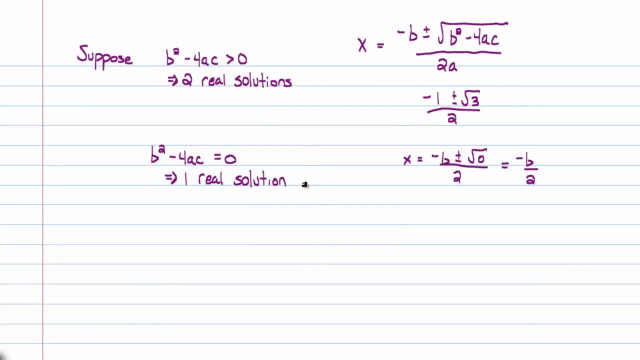 That this, in this case, we would say that our solution has multiplicity too. And the idea of multiplicity does not really come up for a while in a normal intermediate algebra course. 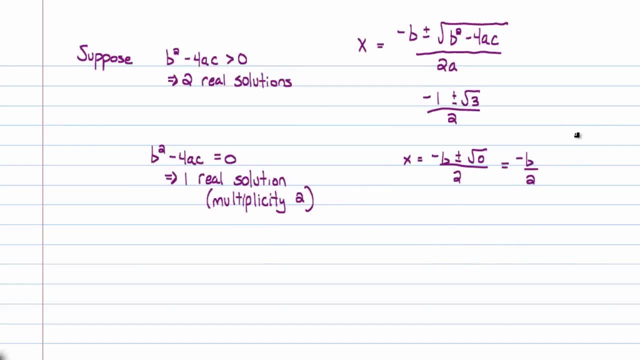 But essentially, it's saying this. That your original quadratic equation... could have factored down to, like, let's say, x minus 1 squared is equal to 0. The solution to this is 1. Right? It seems like we only have one solution, but the fact is we actually have two versions of that one. 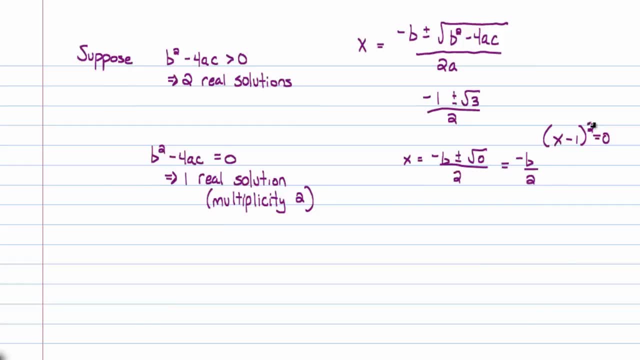 In other words, 1 solves it, but this power says it solves it twice. Okay. 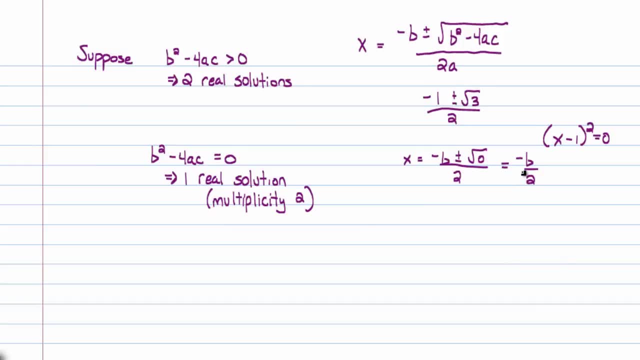 It's not that important right now, but it comes up later on in a course for intermediate algebra. Specifically for graphing, it helps out quite a bit. 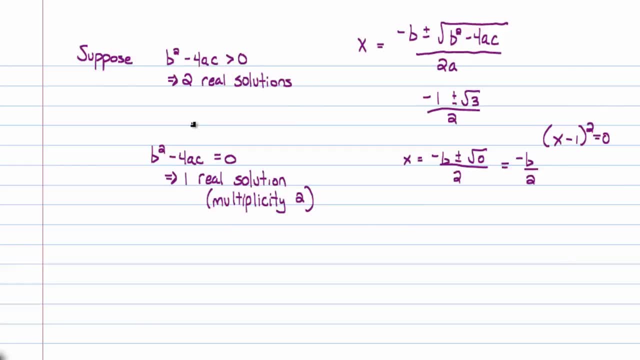 So let's see. We've had the case where our discriminant, b squared minus 4ac, is positive. We get two real solutions. 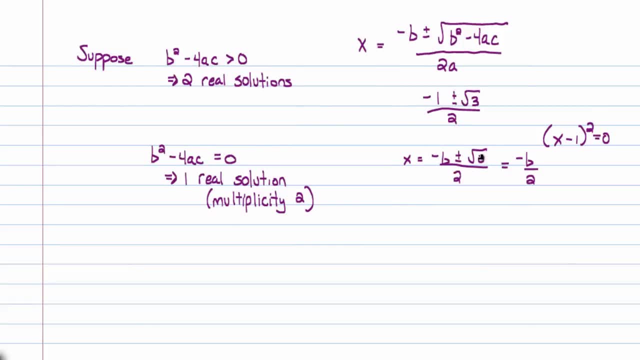 If it's equal to 0, then the stuff underneath the square root turns into 0. So we have one real solution. 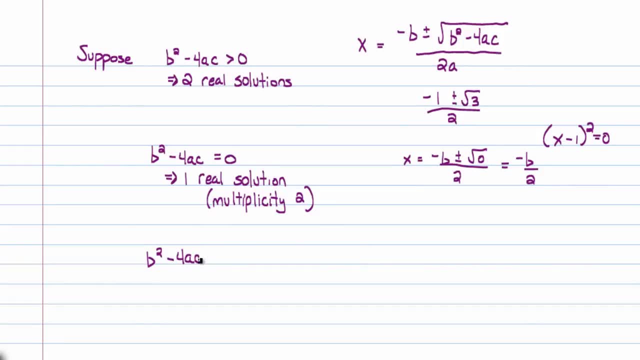 And then finally, if b squared minus 4ac is less than 0, or in other words, negative. 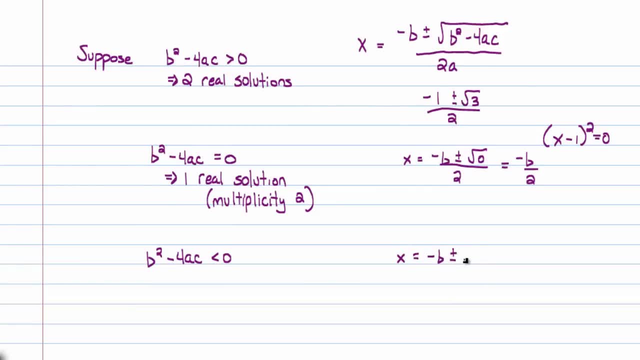 Well then, in this case, we will have some negative number underneath. 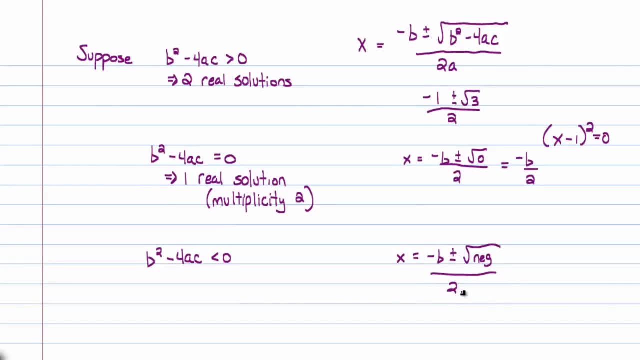 The square root. And so in this case, we will have, oh, I should probably have written 2a there. 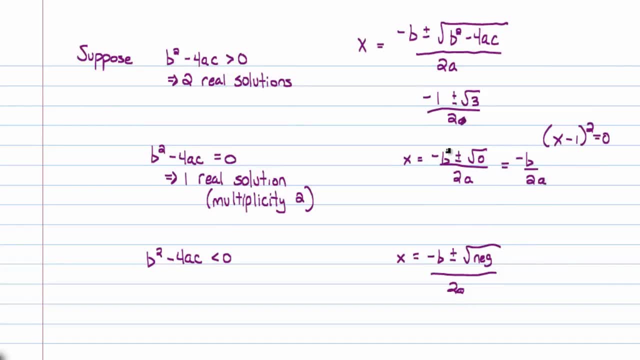 2a there. And 2a down here. Oh, that didn't have 2a. Anyway, sorry about that. 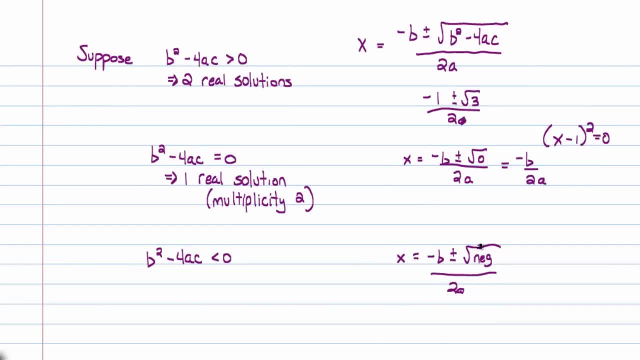 Turns out that if you have a negative underneath the square root, that you have complex solutions. Right? Complex number solutions. 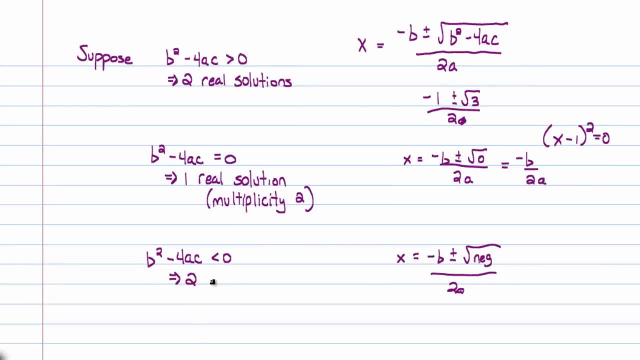 So this implies that you have two complex number solutions. 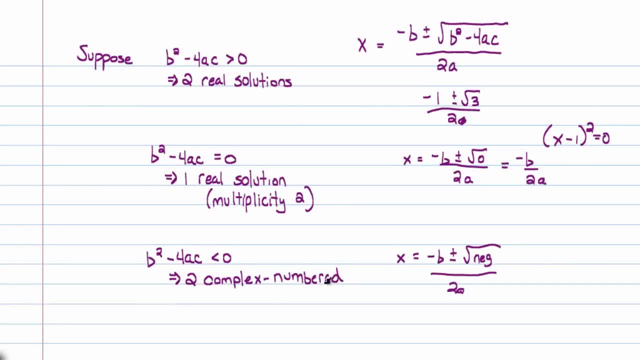 And they will be complex conjugates. In other words, if 1 plus 2i is a solution, then 1 minus 2i is a solution. 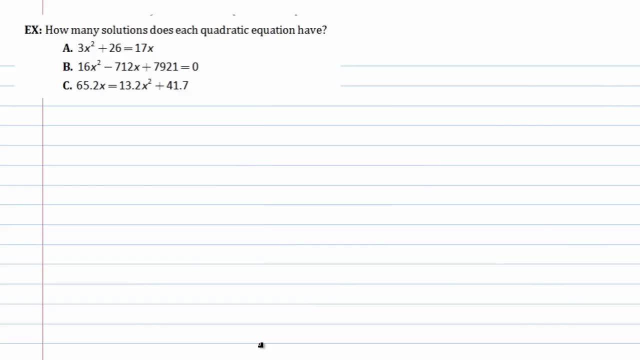 Now, honestly, I've seen some very great uses of the discriminant. It essentially allows you, before you do any heavy calculations, to determine if you actually have a real solution or not. If you're only concerned with having real solutions. 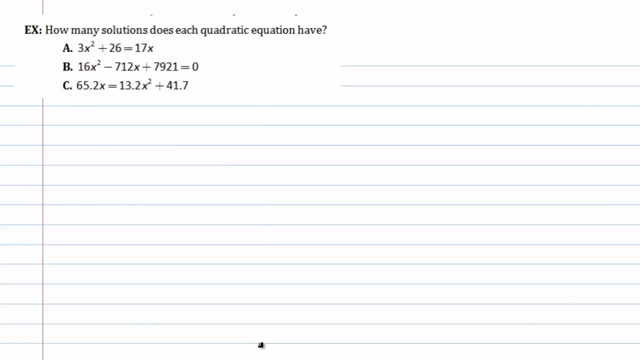 solutions, then it's great to use the discriminant first to check whether or not you even have a real solution. So here's three different quadratic equations, and all we want to know is how many solutions and of which type are our solutions for each of these quadratic equations. 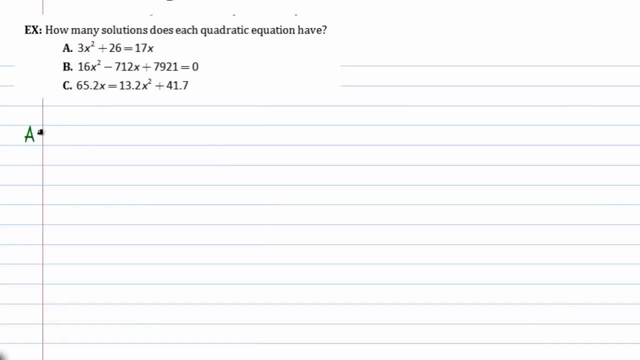 So let's go ahead and look at example A. I have to rewrite this, first of all, to be 3x squared minus 17x plus 26 is equal to zero, and remember the discriminant is just b squared minus 4ac, and that's going to allow us to determine how many solutions there are and of what type. 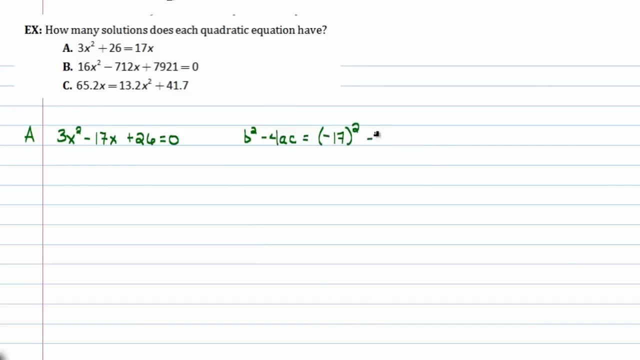 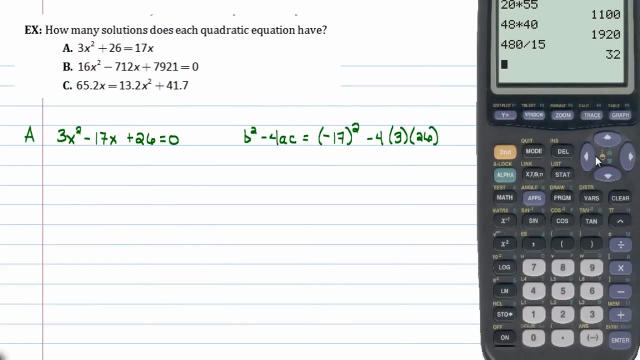 So that's going to be negative 17 squared minus 4ac. 4 times 3 times 26. Now I'm not really too concerned about what the actual number is. I'm more concerned about whether it's positive or negative. So let's do 17 squared, and then minus 4 times 3 times 26. That's a negative number, and that's really all I can do. So I'm going to go ahead and look at example B. I have to rewrite this, first of all, 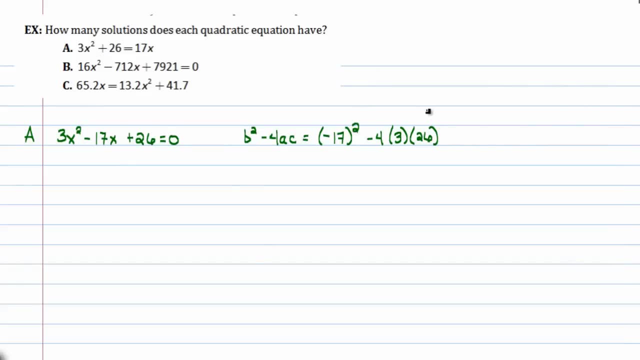 I don't really care what the number is, unless I'm actually trying to solve this, but I'm not really trying to solve it. All I want to know is, is the discriminant positive, equal to zero, or less than zero? And here it's less than zero, which implies we have two complex number solutions, right? And that essentially tells us, if this was for some real application, where we wanted real number solutions, this means that there's no possible way we get real solutions. We have a square root of a negative number. 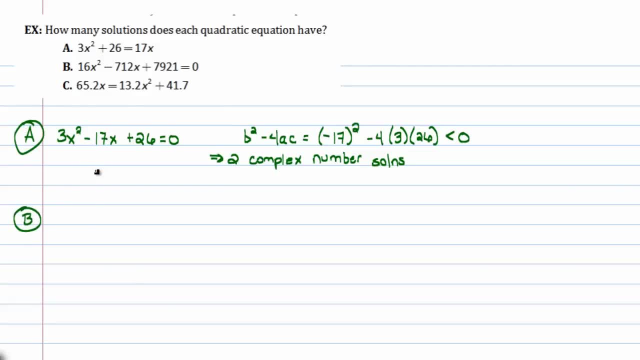 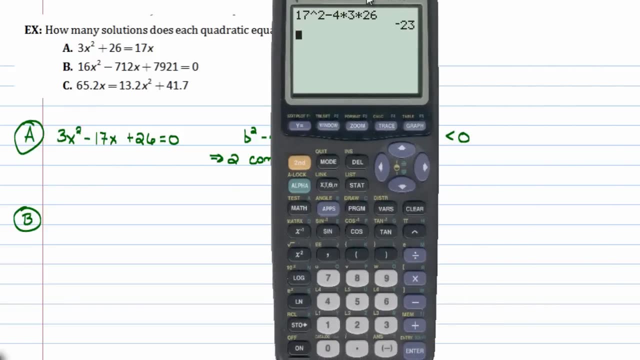 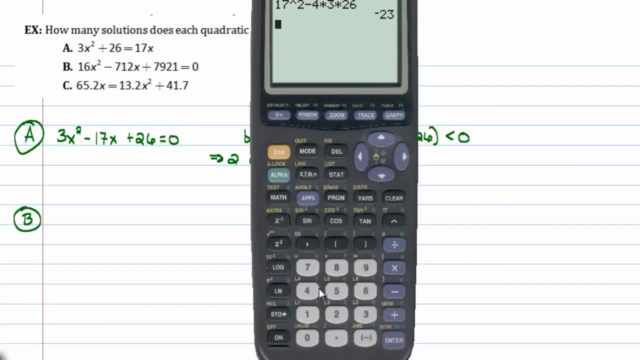